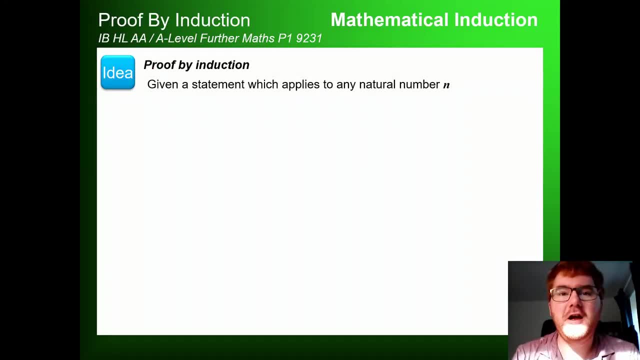 Hello and welcome to another Ginger Math Petition video. It's going to be a little bit different today, so I'm going to work on an IB high level analysis and approaches topic and this is also on the A level further maths paper one 9231 as well for Cambridge and the topic today we're 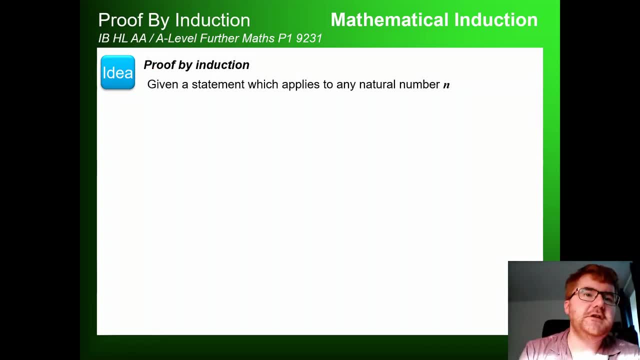 going to look at is mathematical induction, also known as proof by induction as well. In this video we're going to focus on two main questions you could get in the exam, and that is summation. so we're going to look at summation first and then we're going to look at divisibility afterwards. So 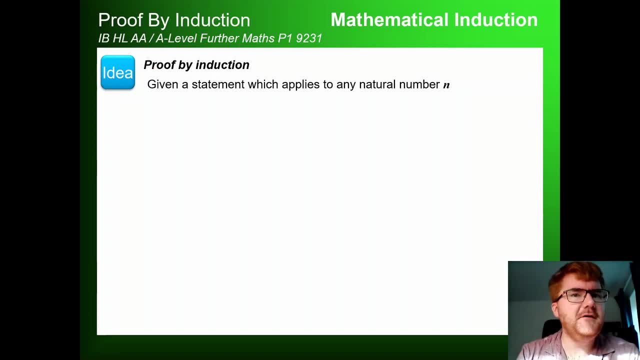 this is a topic that my students have found quite tricky, so I thought I'd do a video on this and go through these two situations. Now, what is proof? by induction, So the definition down below is given a statement which applies to any natural number, so any whole number: n. First of all, we need 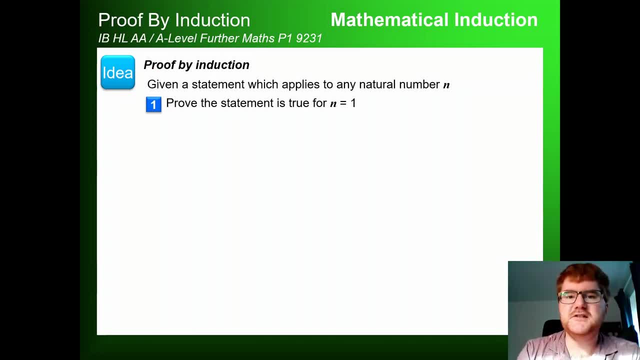 to show that the statement is true. so I'm going to present a statement in a moment. is true for n equals one, then we assume the statement is true for n equals one. and then we assume the statement is true for n equals one. and then we assume the statement is true for n equals one. and then we 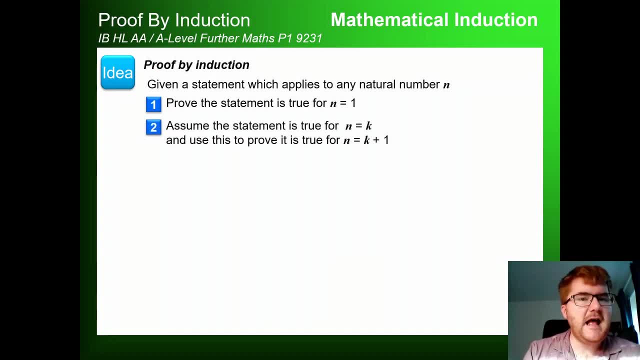 assume the statement is true, for n equals some value k, and if we have that assumption step, then we can then use that to prove it's true. for n equals k plus one. Now, if both one and two are true, it has a kind of domino effect, if you know to go from k to k plus one also works and you. 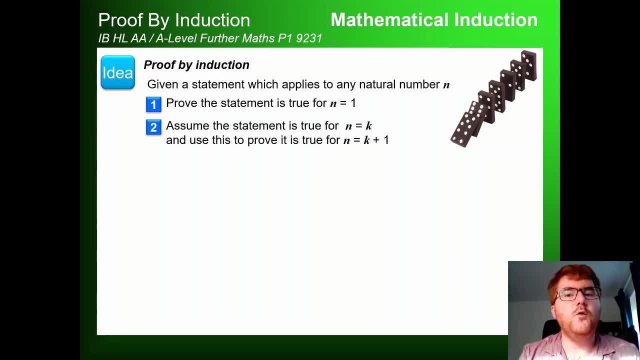 know n equals one works, then it must be true for all values of n. So that's a very quick overview exactly what proof by induction is and why it can be done. So let's go ahead and look at the success of this argument, and then now I'm going to be chewy. The solution I just see that you have is that. 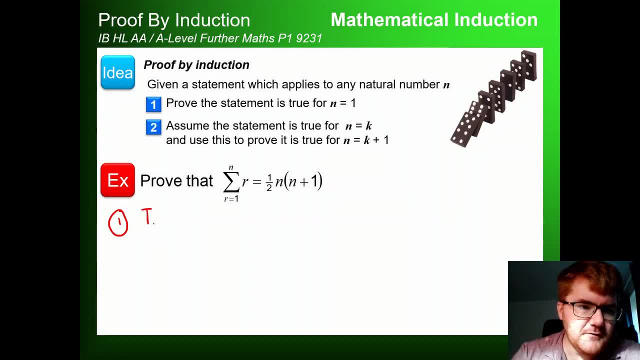 it's true for n equals one. let's just go ahead and introduce that way. if we multiply by, let's say true for關, is what the result will be when we take how many-". and then after that we just pull 2 to 2, writing to what thatmpedge equals. So we need to prove that the result is true for n equals. 1, and so we go through these two steps. the first step is always the relaxing step and then step 2 is We have, we're going to put the other way around. So the first step here is where we say sharpa equals 1 and we're going to do is, we're going to succeed, will create with AutoZoom. we're going to show this is true for n equals one and 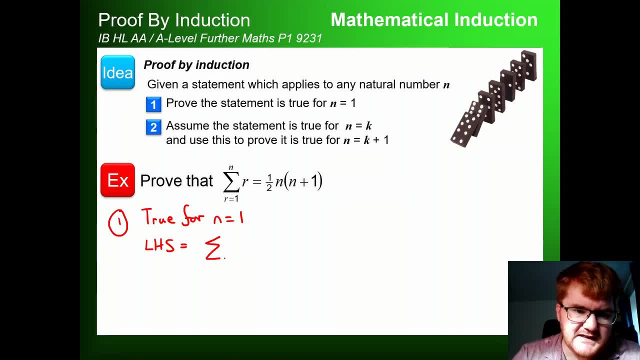 hand side. let's take this here. so wherever I see an n, I'm going to put a 1, so r equals 1 to 1 of r. well, that summation is basically just 1 if we do the right hand side here. and wherever we see an n. 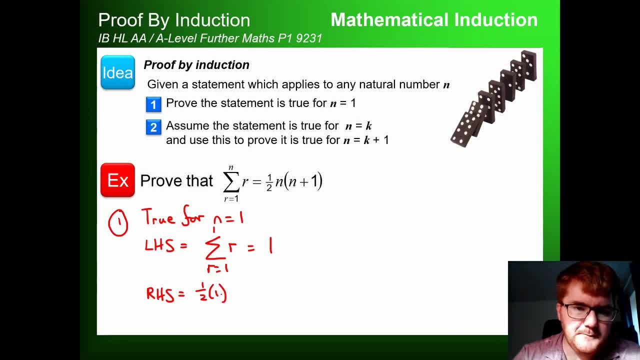 we're going to put a 1, so we get a half. lots of 1 open brackets, 1 plus 1. now hopefully you know that 1 plus 1 is 2, so we get a half times 2 is equal to 1, and notice here that the left hand side 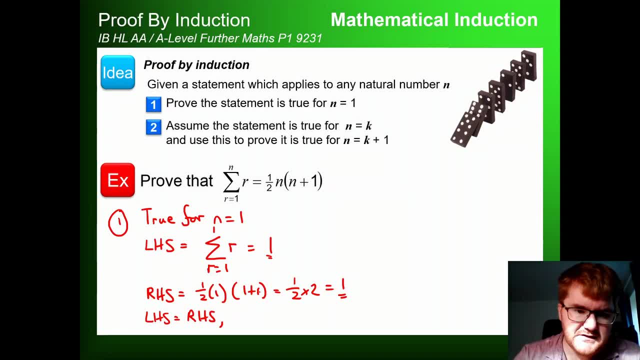 is equal to the right hand side. so therefore I use the three dots. therefore, true for n is equal to 1. so whenever you do a proof by induction, you're going to get a mark or two here just by doing that. it's true for the base step. so true for n equals 1. 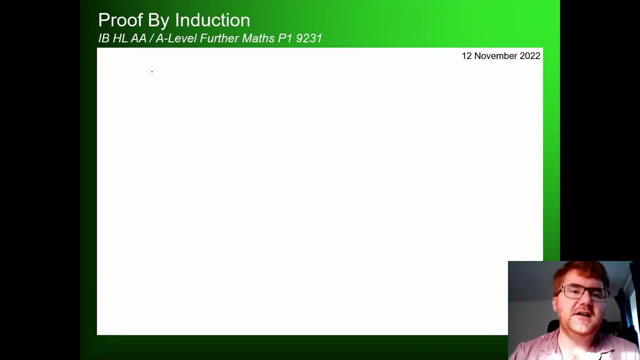 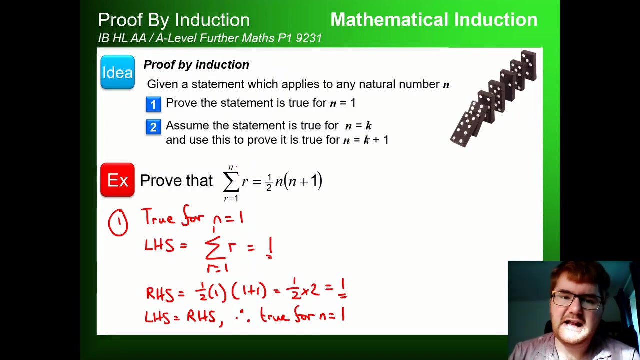 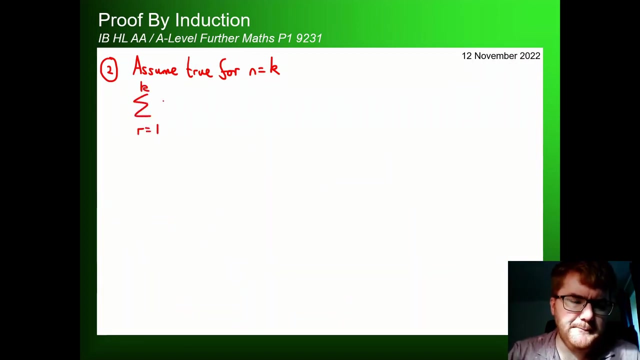 so now where it gets tricky is we're going to do now our assumption step. so we're going to assume it's true for this n equals k, so what I mentioned here. so we go back to here and wherever I see an n, I'm going to put a k. so I'm going to put sum of r equals 1 to k of k. that, oh sorry. 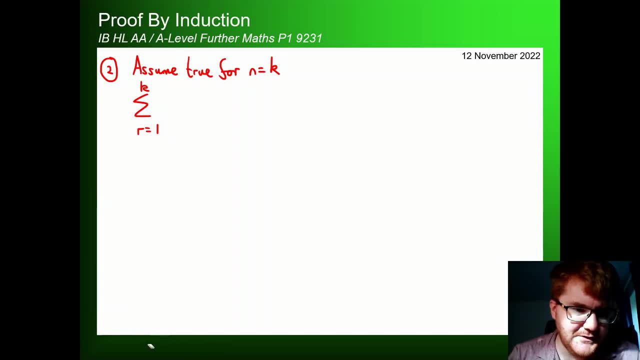 oops, getting ahead of myself, I'm going to write k in a moment. so r and that's equal to a half k k plus 1. so we're going to assume that's true and now we're going to consider. so consider this expression here: so r is equal to 1 k plus 1. 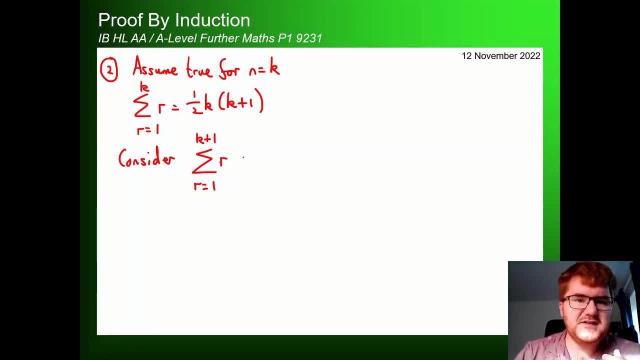 r. now what I'm going to do is write out the sequence. so I'm going to just write out some numbers here. so when r is equal to one, we just get one. when r is equal to two, we just get two. r is three. and notice, we get this sequence and then we're going to get our kth value and then 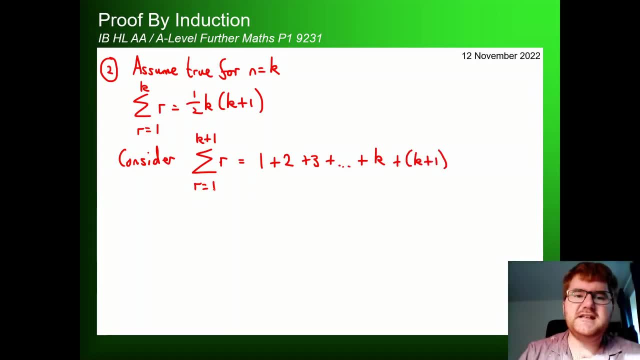 we're going to get the k plus one. so I'm just writing out this very basic sequence here, this basic series here, just so we can actually see what's going on now. what we're aiming for is to basically make this look like this. so let me underline, it takes a bit of practice. we'll do a. 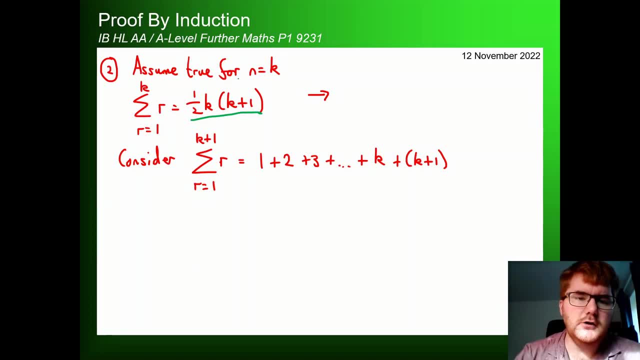 couple of questions today. so we're going to make this look like essentially that, but with k. instead of having k here, we have k plus one. now, what do I mean by that? well, let me just write this really carefully. it's showing what you're aiming for. so wherever I see a k, I'm going to put a k plus one. 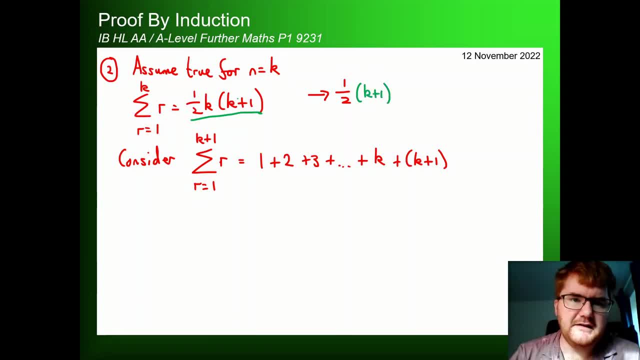 so I've got a k plus one here, and then we're going to have a k plus one, and then we're going to have a k plus one, and then we're going to have a k plus one- and let me now finish this off in red plus one. so that's what I'm going to be aiming for, of course. 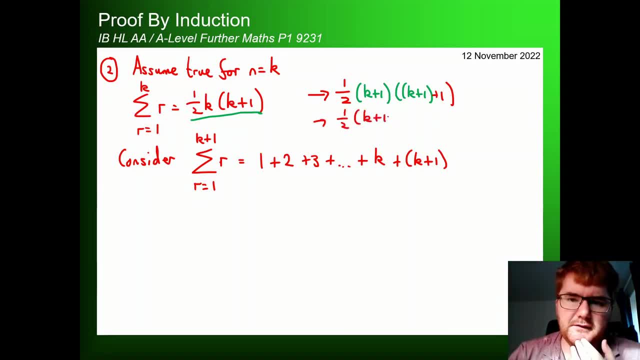 I can simplify this slightly and get a half k plus one, and k plus one plus one is k plus two. so essentially, the induction process summation is: this is what I'm aiming for, so what I'm in the box, and this is not part of the proof, but it's helping to visualize what's going on. so I want to convert. 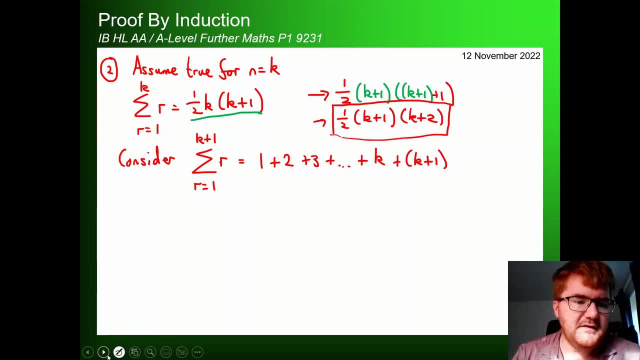 what's down below here into that form. and the only thing I'm allowed to do from the assumption step is convert this section here to what I've underlined in green here, because, remember, that's my assumption, that this is true. so I can change that to a half k k plus one, so I'm allowed to. 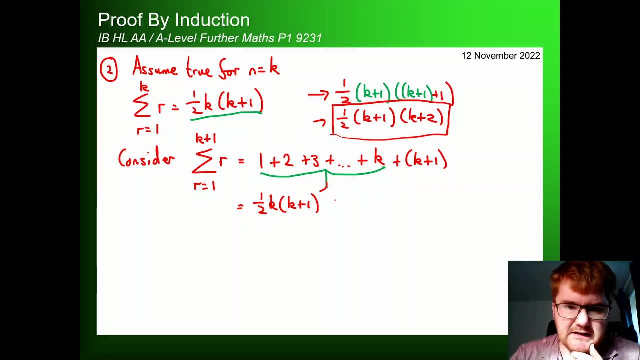 change this to this, because that's my assumption. don't forget, we've also got the k plus one here, and what I want to do is this expression: I want to change it to look like this: the box. now the thing is to have faith in the process here. you know it's going to work because 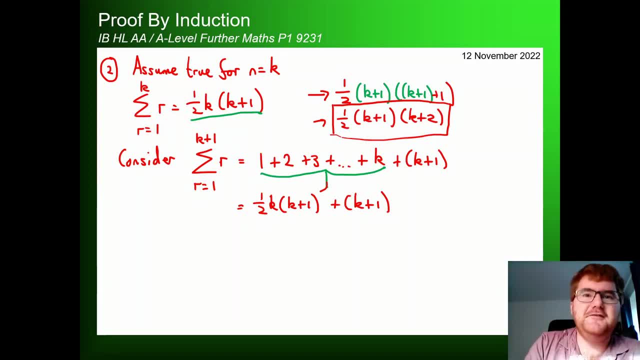 you're told. prove that I'm not going to try and trick you and give you something that doesn't work. so you know, you have to get to that in some stage now. my thought process here is: well, I need a half and I need a k plus one, specifically the k plus one. so the first step I'm going to do here is: 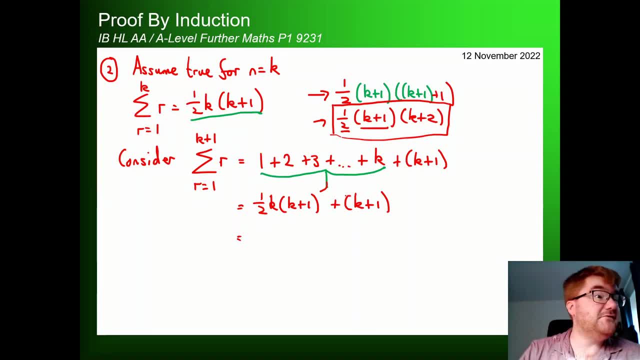 actually going to take a factor of k plus one out of both, factorize into a single bracket, essentially. so I've got k plus one and then I work backwards. so what do I multiply k plus one by to get a half k k plus one? well, just, 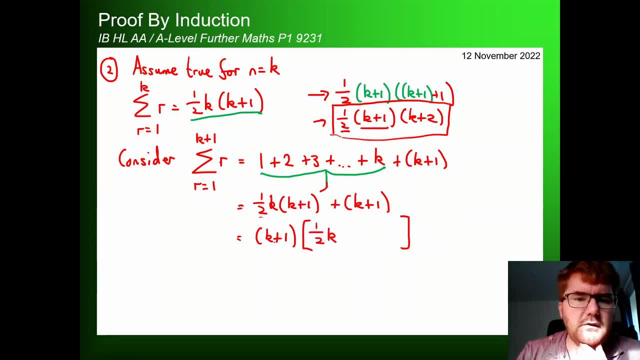 a half k. and what do I multiply k plus one by to get k plus one? well, just one like. so, again, it's not entirely the form that we want, but what we can do at this point is take a factor of a half out as well. so what I'm going to do now, from this square bracket, I'm going to take a factor. 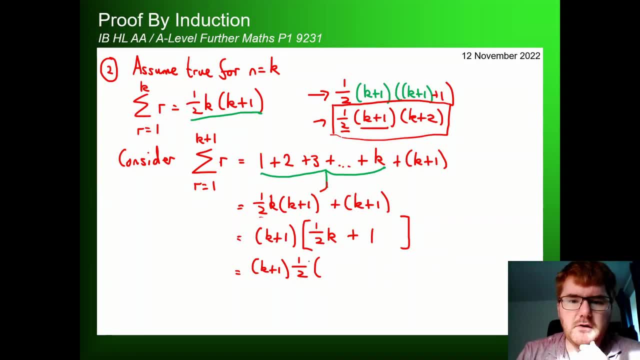 of a half out and do the same process. so what do I multiply a half by to get a half k? well, k. and this is where it's nice and sneaky. what do I multiply a half by to get one? well, two. and notice, because multiplication is commutative, you can move it around, we can just put this in the order. 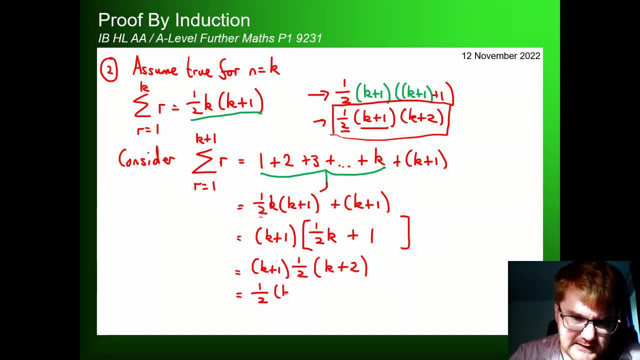 that we want. so we get a half k plus one k plus two. notice, it's exactly the same as the box that we have here now. what I'm going to do at this point is I'm going to take a factor of a half out and multiply it by two. so what I'm going to do at this point is just make it really obvious to the 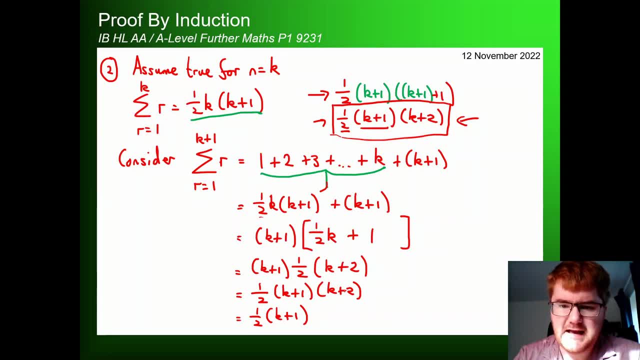 examiner. I'm going to replace the k plus two here with the expression I did before, k plus one plus one, to make it look like what I've just done here and because we've actually got it in that form that we wanted. we can then say: it is true: for n equals k plus one, and because we've done those two steps. 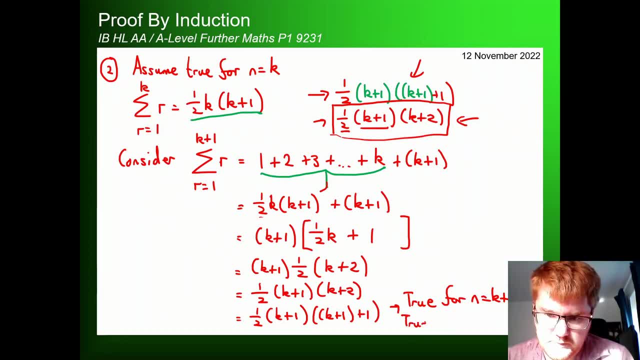 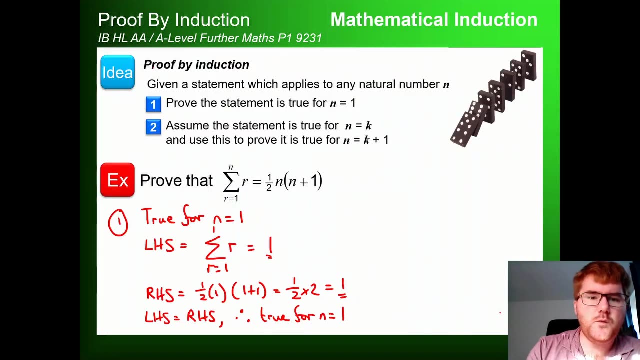 we then know. it is then true. now you can use this symbol here for all, so for all: n as a natural number, so like this. okay, so that's the key process of proof by induction. so first of all we do our base step here. that's really important. and then step two. 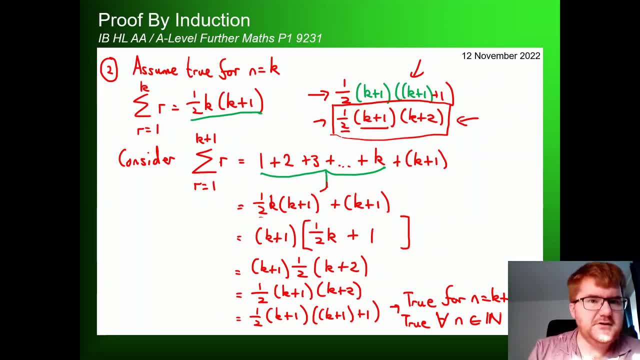 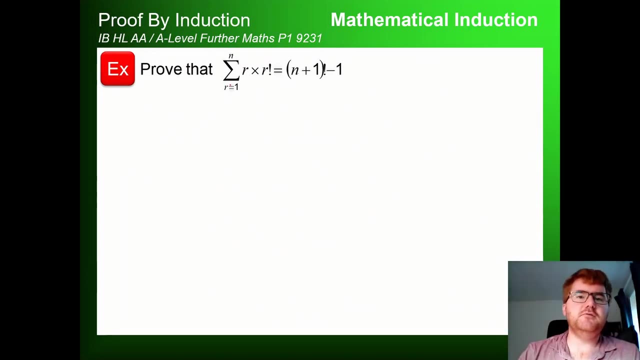 we assume it's true, for n is k. so we just substitute k where n was, and then we consider the k plus one version and then try and make it in that form. now that just does take a bit practice. we're going to do a few examples today. right on to example two here. so we're going to 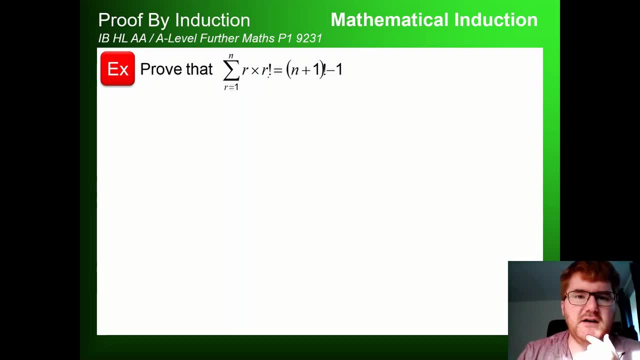 show that this expression of the summation here, r plus r times r, factorial going for r is one to n- is the same as this. again, we follow that same process. remember this exclamation mark. we call it a factorial in mathematics. just remind you what that is: three factorial here is the same. 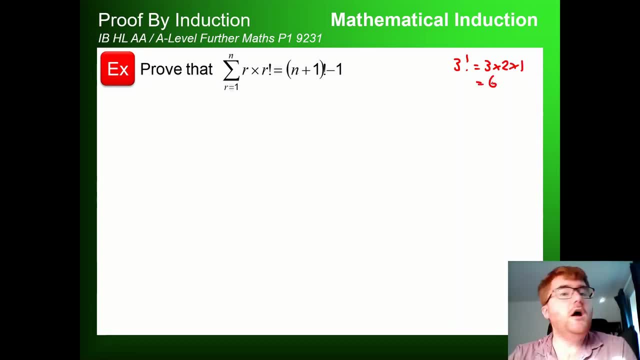 as saying three times two times one is equal to six. hopefully you've already seen that on the course that you're doing. so the first thing we need to do is establish, if it's true, for n is equal to one. so that's always the first step, the fairly straightforward step here. 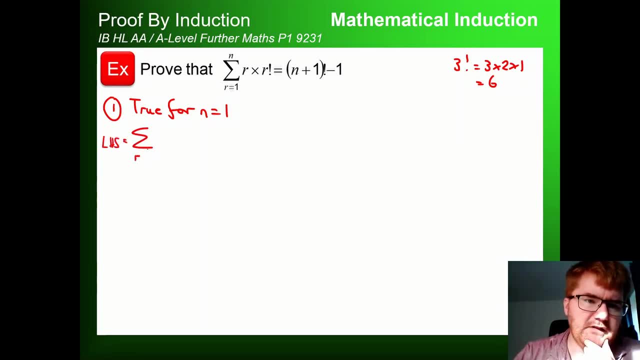 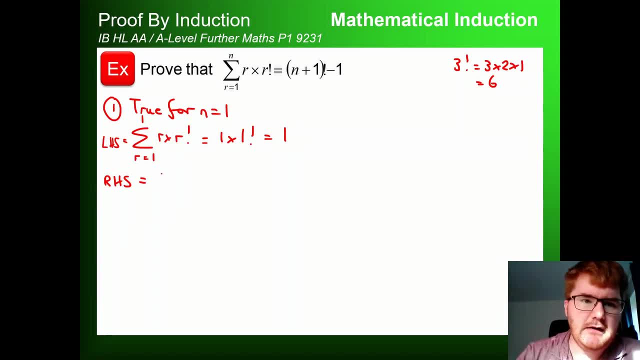 thing here we do the right hand side. so that's going to be one plus one factorial minus one. one plus one is two. two factorial minus one. that's just going to be equal to one. so therefore the left hand side is equal to the right hand side. so true, for n is equal to one. so again you. 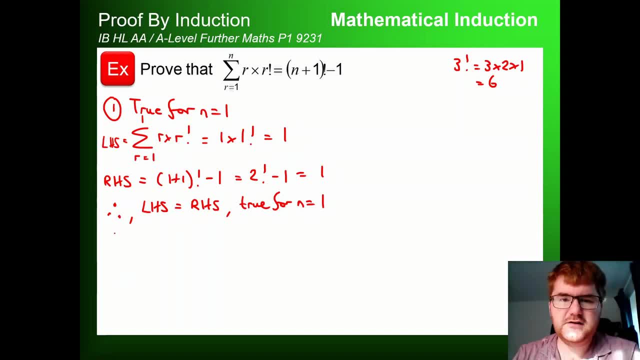 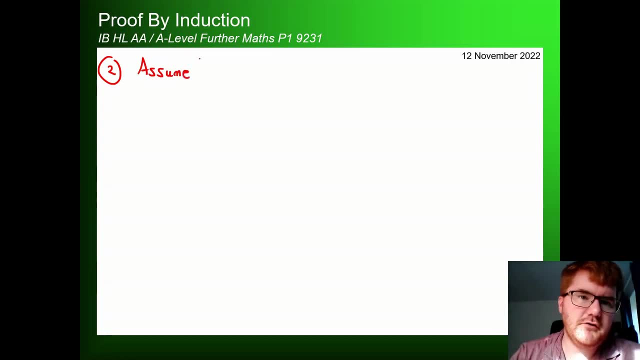 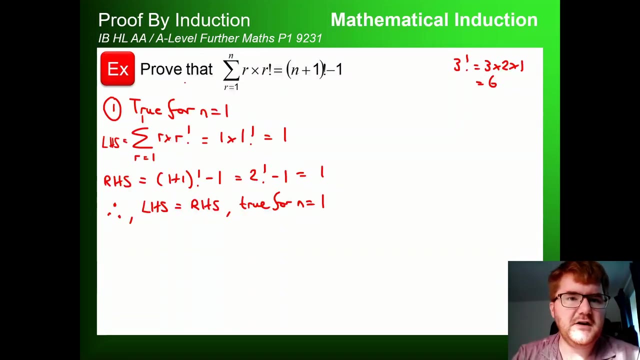 always have to do that base step. now this is where it gets tricky, so let's do it on a separate slide here. so I'm going to assume true, for n is equal to some k. so basically we're going to copy out the left hand side here. wherever I see an n, I'm going to put a k, so we get the r equal to 1. 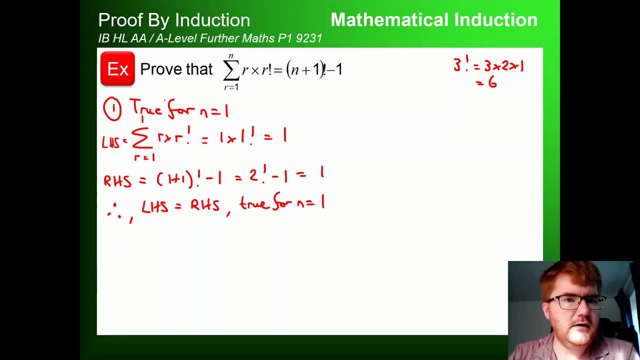 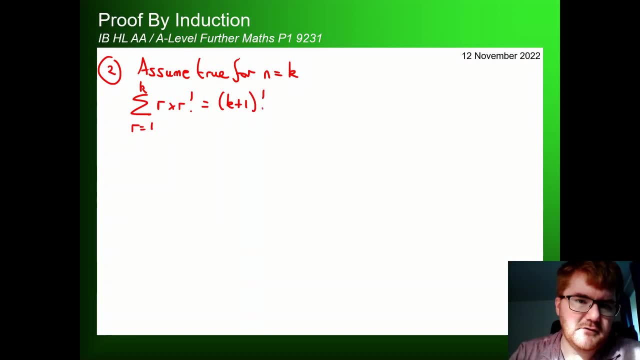 to k r times r factorial, and that's equal to k plus 1 factorial minus 1. so we're assuming that's true and now we need to consider this term here. so r is equal to 1, k plus 1, now r times r factorial. okay, so when we substitute 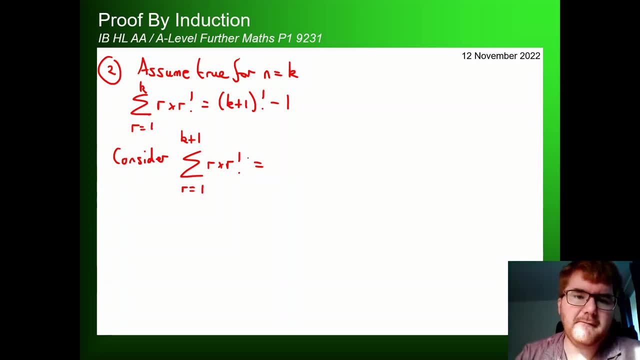 numbers again. we're going to have to do the back hand side, so we're going to have to do the back in to see what's going on. so, first of all, 1 times 1 factorial is just 1, 2 times 2 factorial, that's. 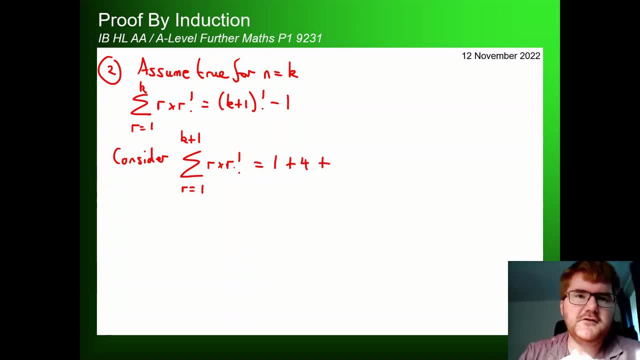 going to be equal to 4, 3 times 3 factorial. this is not necessary, but just so you can visualize. so, 3 times 3 factorial- well, remember, 3 factorial was 6, 6 times 3- is 18, dot, dot, dot. and then we've. 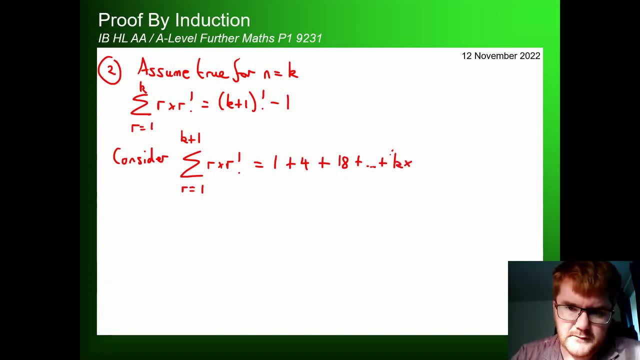 got the kth term, so k times puts in brackets k factorial, then plus the k plus 1 term, so k plus 1 times k plus 1 factorial. now before we get into the induction process here, I always like to see, to visualize what I'm aiming for. so I take the right hand side. wherever I see a k, I put a k plus. 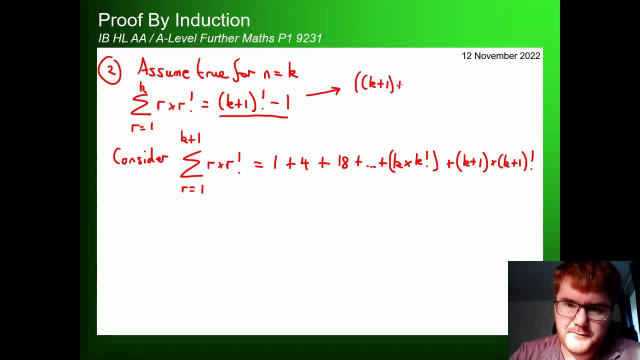 1, so this will look like k 1 plus 1 plus 1 factorial minus 1. so what I'm looking for- and this is what I want to achieve- is this expression here. so I've got the expression down below and I want it to look like what's in: 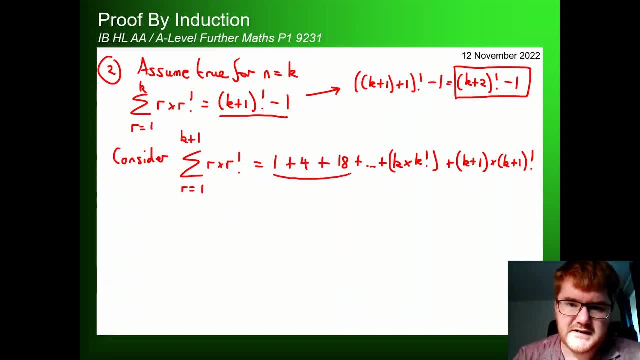 the box and the only thing we're allowed to substitute here. so we take the sequence up to k. we know from the assumption step it's equal to k plus 1, factorial minus 1. so I'm going to replace this with k plus 1, factorial minus 1. and then don't forget the k plus 1th term. so plus k plus 1, k plus 1. 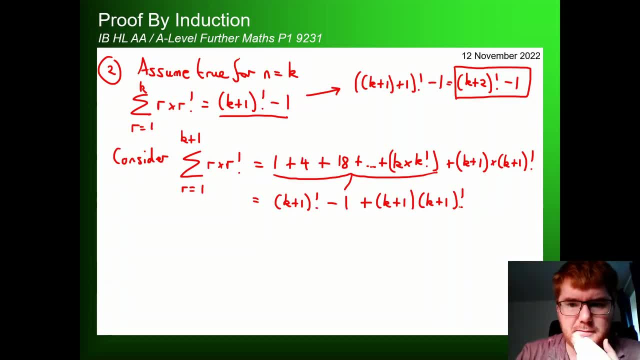 factorial. okay, so this is a little bit trickier to work with. here again, as soon as you look at a question like this, the first thing I generally want to try and do is factorize. now I want a minus 1 at the end, so I'm going to move this around slightly, so I'm going to get a k plus 1 factorial. 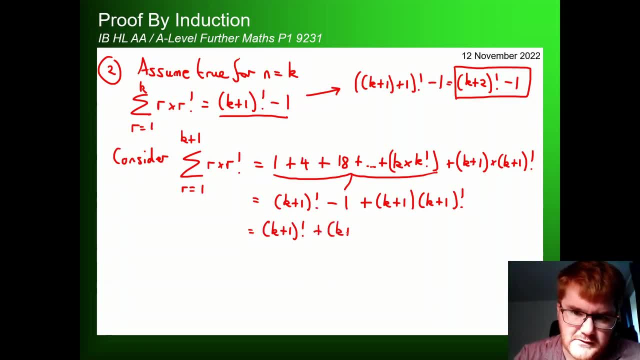 I'm going to just move the terms around because I know whatever happens, I need a minus 1 at the end, because that's in the question, and at this point I'm going to take this part of the expression and factorize so I have a k plus 1 factorial in common. you trust the process, so k plus 1 factorial is in. 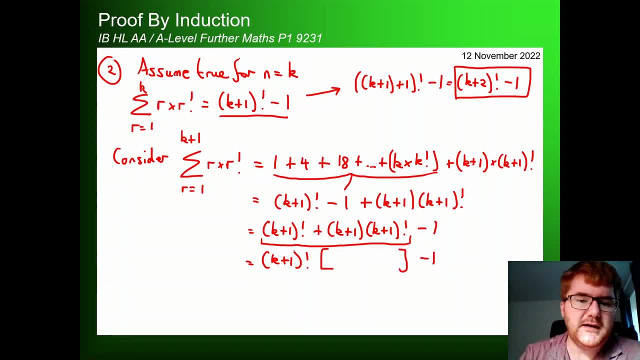 common, and now I work backwards. so what do I multiply k plus 1 factorial by to get k plus 1 factorial just 1? what do I multiply k plus 1 factorial by to get k plus 1 factorial just 1? multiply k plus 1 factorial by to get k plus 1 times k plus 1 factorial. Well, the only thing. 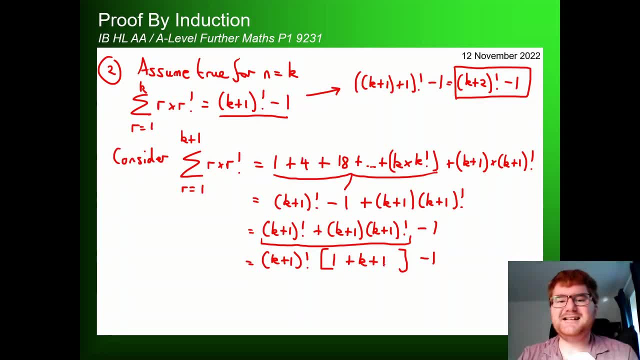 different is the k plus 1.. You're probably thinking at this point I'm not really getting anything that's looking like what I want. Trust that process. So we collect things up- k plus 1 factorial, and if we simplify this, we get k plus 2 minus 1 and surprisingly we're almost there with 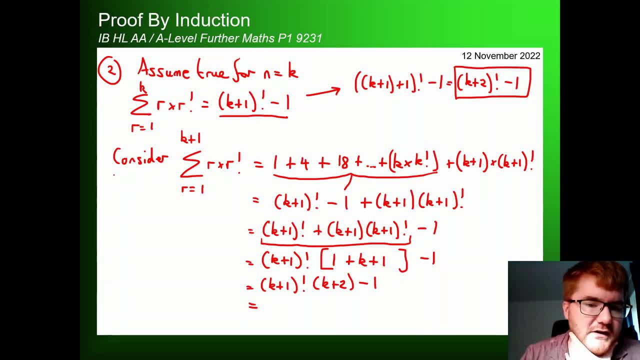 this particular question. Let me give you some numbers to visualize what's going on. So say, I've got 4 factorial and I times it by 5.. Well, what I could do is rearrange this slightly: 5 times 4 factorial. Now remember what factorial is. it's just 4 times 3 times 2 times 1, and notice this. 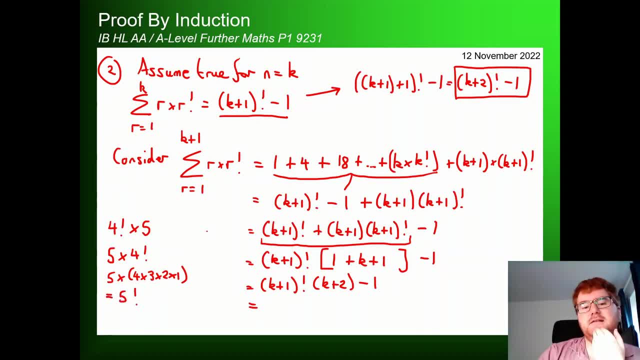 is the same as just 5 factorial. It's just kind of sneaky, particularly if you're not used to using factorials. So because I've got the total number of factorials, I can just do this. So I can just change this directly to k plus 2, factorial minus 1.. So I'm exploiting this idea that if I've got the 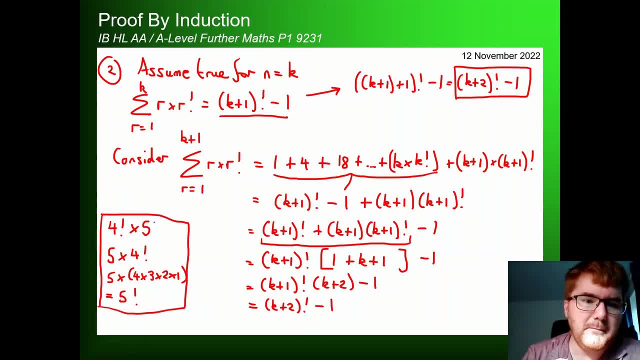 next term, and I'm multiplying by it. you can actually just change this into factorial. It's a nice little sneaky trick. I've left there on the left hand side for you, and then we get exactly what we want in the box. Now, just to make it clear to the examiner, I would then just write this as k. 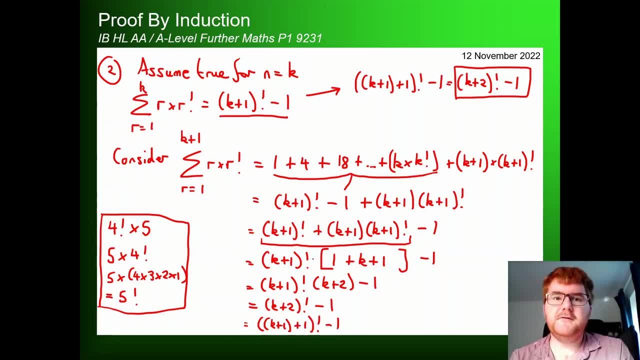 plus 1 plus 1 factorial. So it's very clear that I've got that k plus 1 expression. So from that I then know that it's true for n equals k plus 1 and therefore true for all n. Do we have any conditions on what n is? I assume? 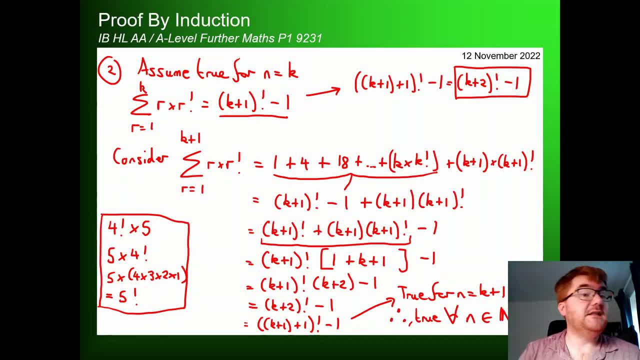 it would also be the natural numbers as well, just like the previous example. So hopefully you've seen from this second example here. So this is a pretty simple way to get the answer And it's actually really easy. You just need to trust the process and just keep working your way through and you will get to the right answer at the 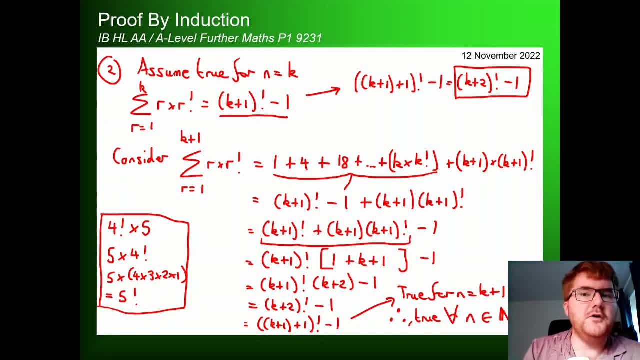 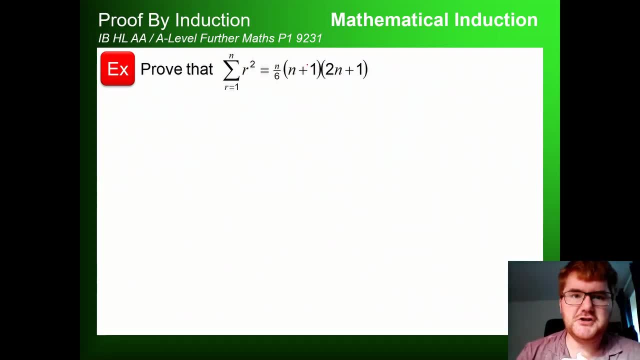 end. It might take you a bit longer if you take a slightly different approach, but you will always get there. Just keep at it with the algebra and make it look like what you're aiming for. Okay, and on to the next example here. So I want to prove this summation here is equal to this expression. 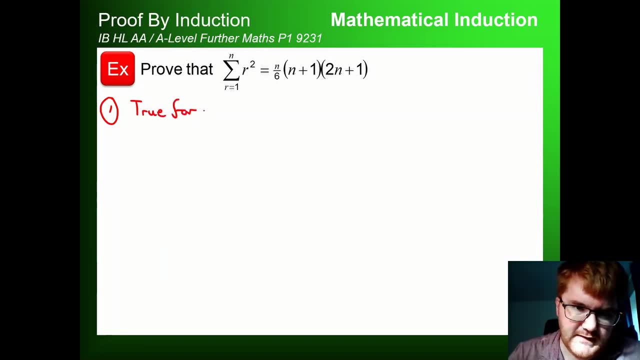 here Again, we go through two steps. So first of all we want to find if it's true for n is equal to 1. to 1, so left hand side, against the same process we just keep going through. so the R is equal to. 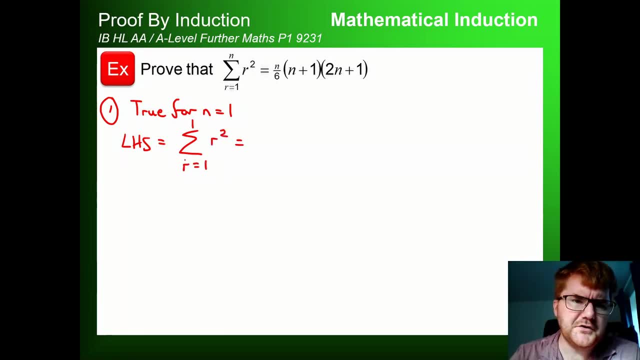 1 to 1 R squared. well, just 1 squared is equal to 1 right hand side. well, we get 1, 6, 1 plus 1, 2, lots of 1 plus 1. if we work through that, we get a 6 times 2. 2 times 1 is 2 plus 1 is 3, so 2 times 3. 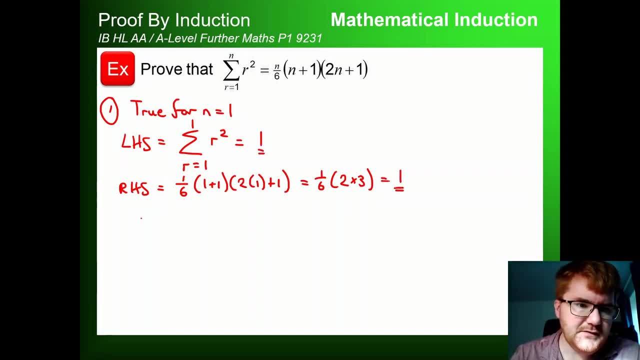 and that's going to simplify down to 1. so our left hand side is equal to our right hand side. so therefore, true, for n is equal to 1, like so? so we've got our base step done. now it's time for the fun part of the game. so let's get started. so let's get started. so let's get started. so let's. 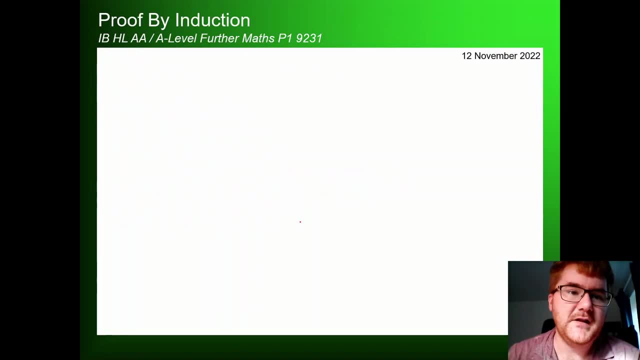 start, which is the assumption, step and go from there. so we go and assume the deep breath at this point. so assume that this sum from R is equal to 1 to K. R squared is equal to what we have in the question. so K over 6- see, the algebra is going to get a bit more messy here- K plus 1 and 2. K over 6. 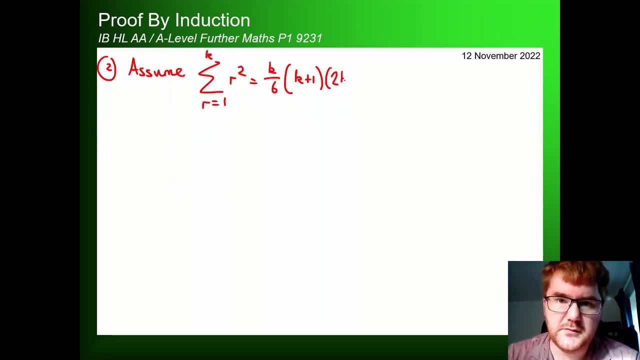 K plus 1. so we're assuming this and then we consider the again. you don't have to write this part out, I always like to, just to see what's going on. R squared- this is just a square numbers here. so we've got 1 plus 4 plus 9 plus K squared, plus K plus 1, all squared. now let's think about what. 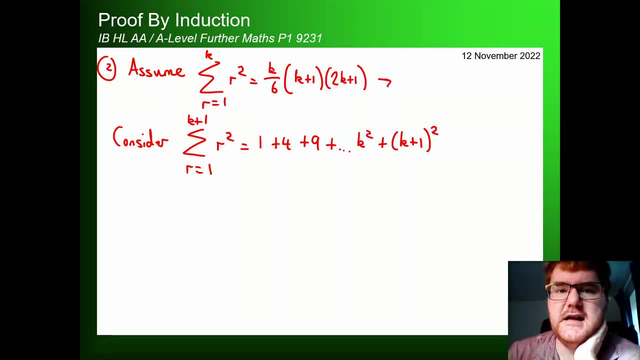 we're aiming for here. so this is a bit more complicated to explain. so let's go ahead and express. so the K becomes a K plus 1. so we get K plus 1. we want one extra to this. that gives us K plus 2. and if we're doing a K plus 1 here, just be very careful. here we're actually aiming for 2 K. 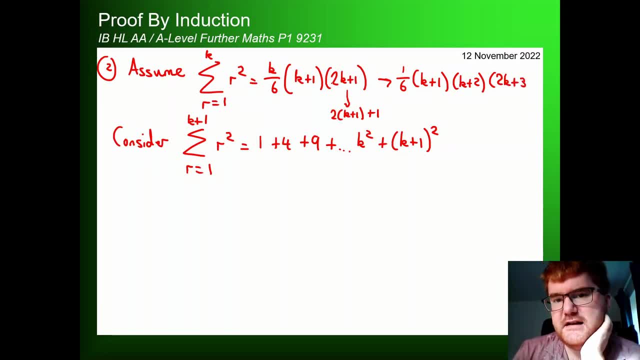 plus 3. so remember: the K plus 1 gets times by 2 and then add 1. so this is what we're aiming for, this fairly complicated looking expression, and this is what we have, and the only thing that we're allowed to do here is replace that with our assumption. so we get K over 6, K plus 1, 2 K plus 1. 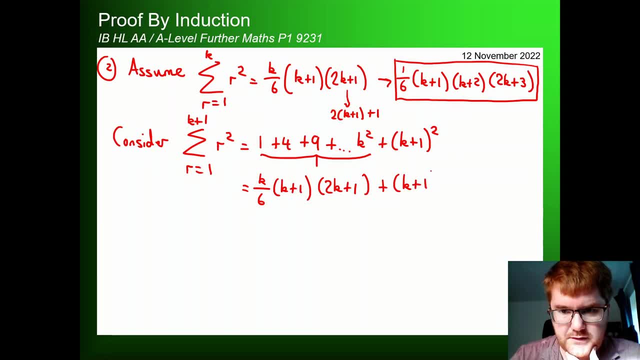 plus K plus 1: squared okay. so the first step to consider here is: what factors do we actually want here? well, we can take K plus 1 out. we can actually take a sixth out if we're careful. so one of the first things we can do is we can take a sixth out, and we can actually take a sixth out, and we can. 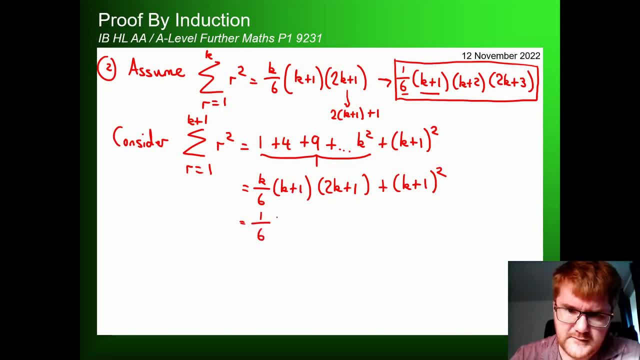 do here is actually take out one sixth and a K plus 1, because they are both sort of in common. well, the number is not in common, but we'll see how we deal with that now. so if we then work out our square brackets here. so what do we multiply this by to get the first term? well, the sixth is: 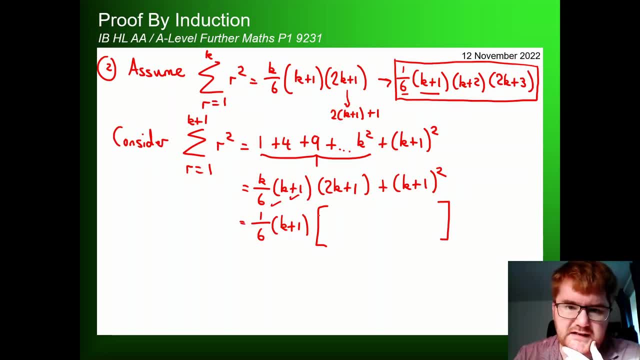 there, the K plus 1 is there, so we're left with just the K and the 2 K plus 1. so we're left with just the K and the 2 K plus 1. so we're left with just the K and the 2 K plus 1. so we're left with 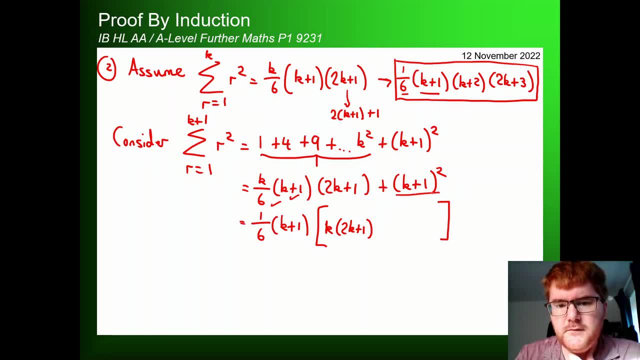 that in, and then we look at the second term. so what do we multiply this by to get that? well, we need a 6, which is the thing to watch out for. remember, 6 times a sixth is 1. remember, we've got a kind of coefficient of 1 here. and we also need to multiply it by a K plus 1 as well, because 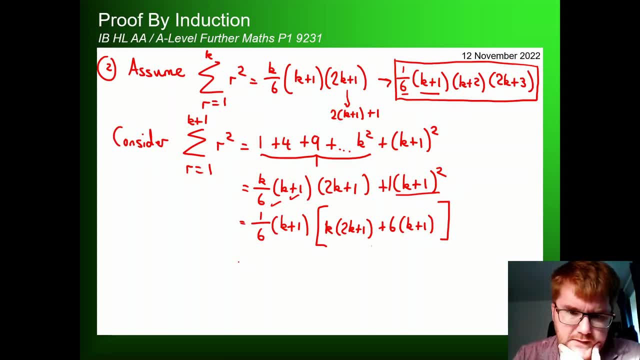 K plus 1 times K plus 1 is K plus 1 squared. so we're making progress here. we've got the first part of the expression. we just need to now make sure that this square bracket does equal the last two terms. we expand the bracket, we get 2 K squared plus K plus 6, K plus 6 if we simplify that down. 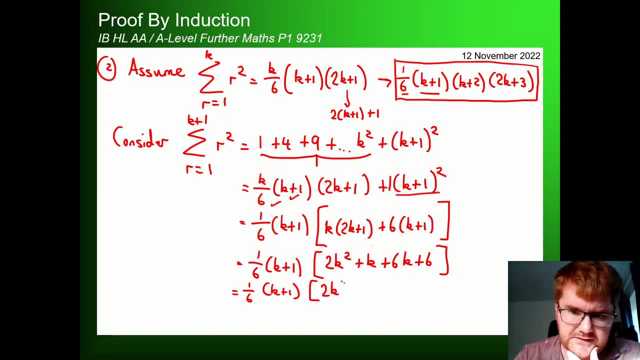 we get 2 K squared plus 7 K plus 6. okay, I think we're making progress here and if we work through it again, I'm going to get our initial term for K plus 7 squared. so at this point you can see that we've got our dot in plus 1 K squared plus 6 squared squared does equal the last one squared. 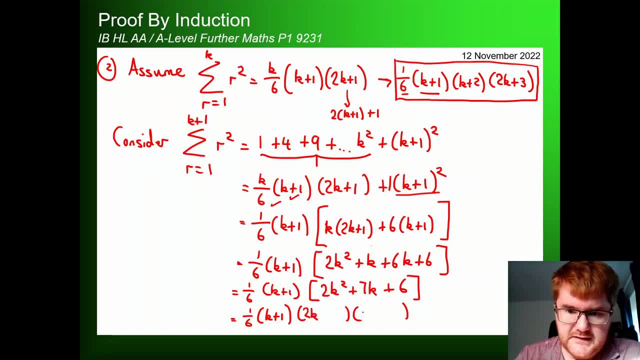 so that gives us 1 plus 2 squared plus 1 squared squared. so in some cases this would be left. that's the difference. so there's not much difference in terms of, ultimately, what's going on. the ridiculous thing we're requesting in this case is if we, if something goes wrong, it tear. 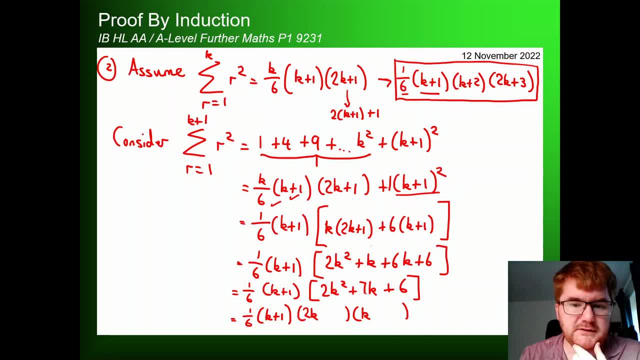 apart the bracket, we wouldn't want that matter here. the 3 in 1- and we also need tootsy interrogation. that's going to be ok, Ziel noi, we don't need this anymore. so let's say: we want every other value in our system. we want the value on the other side of the table. that's going to be the. 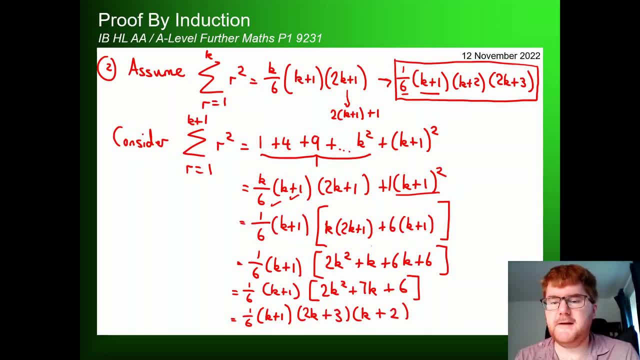 same here. we like to do thing like Tr roof Hold on there. a second time it's going to take 7 out in 2. is that 6 squared squared, or 2 and 2k plus 3 goes there again. I always do this mentally in my head here. so 2k times 2 is 4k 3. 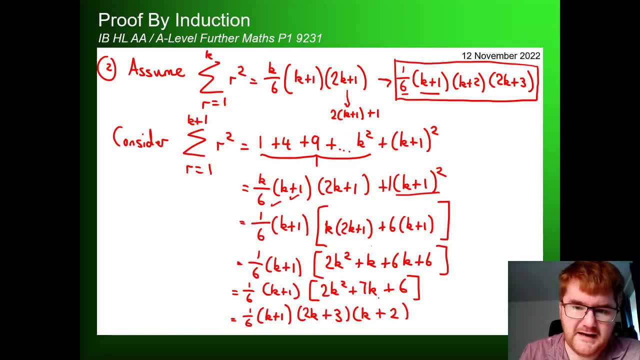 times k is 3k. 4k plus 3k is 7k. okay, I get that term there and notice we do get to the expression that we wanted. so all we need to do is move this around slightly. now for the examiner I'm going to 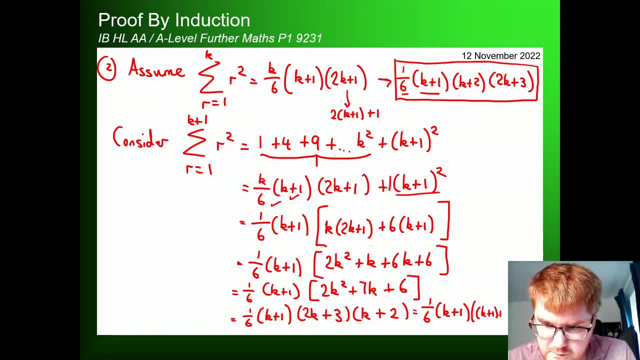 make k plus 2, this kind of weird form of k plus 1 plus 1, to show that it's basically this with a k plus 1 inserted, and then likewise back factorize this as well to get. you're not going to see this, so let me pop this over here. so I'm going to put this over here. so it's 1 6th k plus 1. 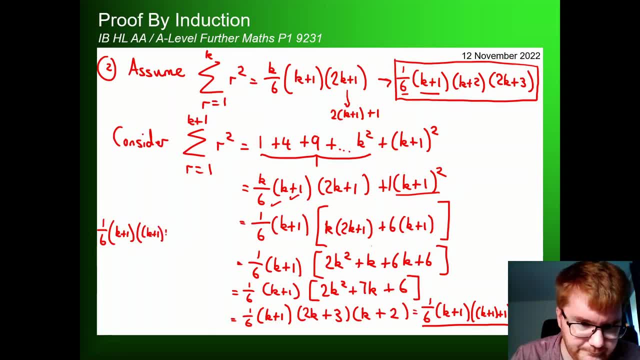 k plus 1 plus 1 and then two lots of k plus 1 plus 1, so we do get it in the form that we want. therefore, it is true for n is equal to k plus 1 and therefore for true for all values of n. again, i'm going to assume this is the natural numbers here. 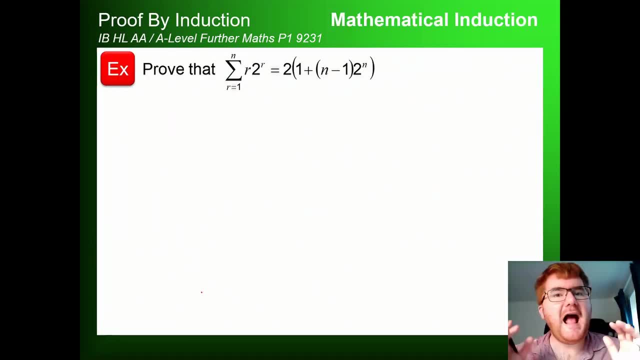 and just the positives. okay, so have a go yourself. i put a question for you in front of you, so give this a good 10-15 minutes. see if you can actually prove, using mathematical induction, that the summation on the left hand side is equal to the expression on the right hand side. need to pause. 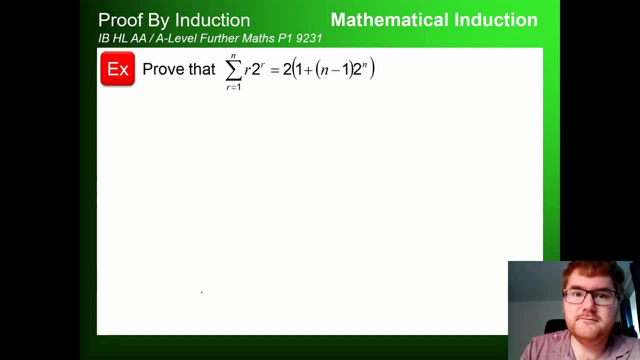 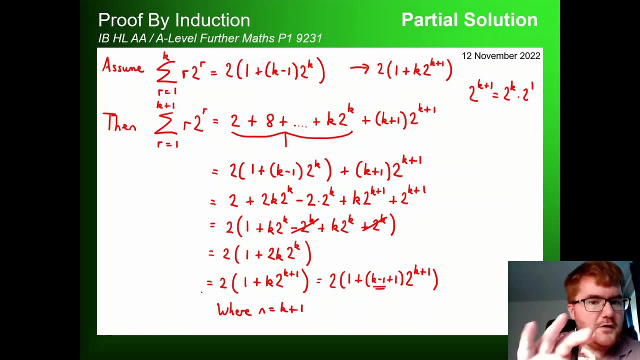 your video. this is the time to do it. okay, and if you got stuck on that assumption step, i've put the work in front of you there so you can go through the partial solution- probably the part of the solution that you do need to check carefully again. this is only one way of doing. 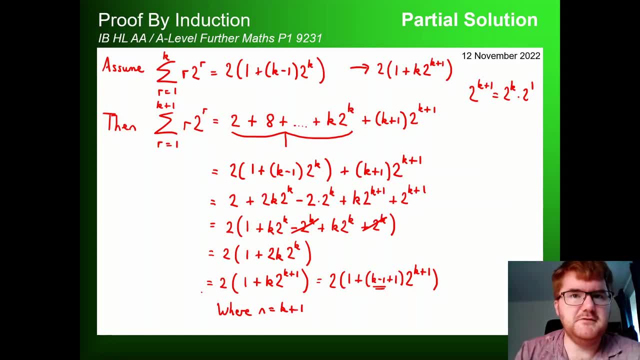 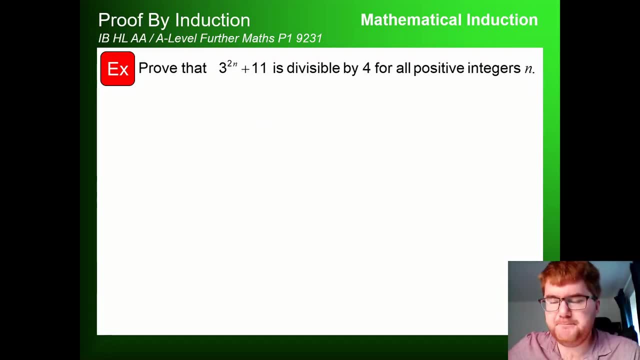 it. there could be more than one way of getting to the correct answer here as well. okay, and on to part two. so we're going to look at some divisibility questions here, again also very typical on both the ib high level aa course and the a level further maths paper one. 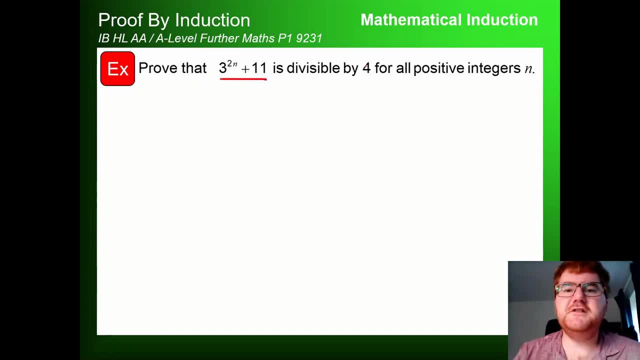 so we're going to prove that this expression here is divisible by four for all positive integers: n, so all those natural numbers, and again we approach this in the same way we did with summation as well. so first of all we want to establish that this is true, for n is equal to one. 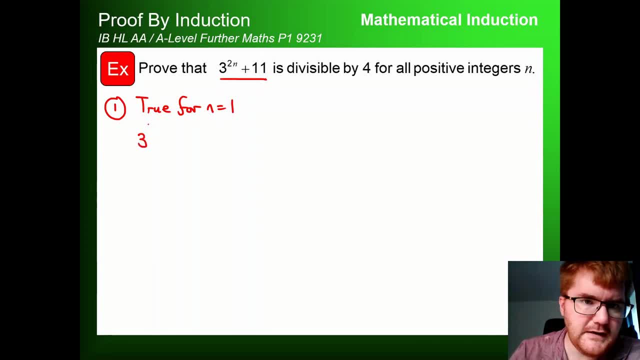 so we're going to substitute one in so three two times one is two. so we're going to substitute one in so three two times one is two. so we're going to substitute one in so three two times one is two plus 11, so that's going to equal 20, and again i'll show you that's divisible by four by just. 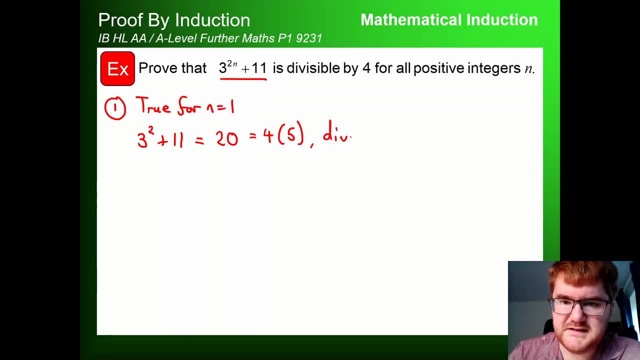 taking a factor of four out, therefore, this is divisible by four for all natural numbers. so again, we always do that base step and just check for n equals one that it works. now, the way we approach the assumption step is the following: so we assume, so this is slightly different in terms of format. assume: f of k is equal to three, to the power of two k plus 11. 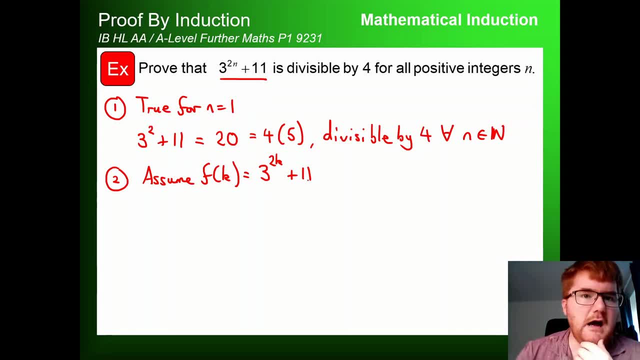 so i take that expression. wherever i see an n, i'm going to put a k, and what we're going to consider here, using some function knowledge from earlier courses, is we're going to work out f of k plus one okay, and you can probably see where we're going to aim with once we found an expression for this. 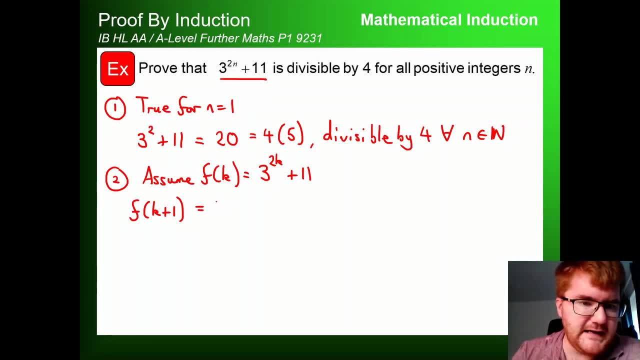 so i take this expression wherever i see an n, i'm going to put a k, and what we're going to consider here, using some function knowledge from earlier courses, is: we're going to put a k and what we're going to consider a k, i'm going to put a k plus one. so get three to power of two brackets: k plus one. 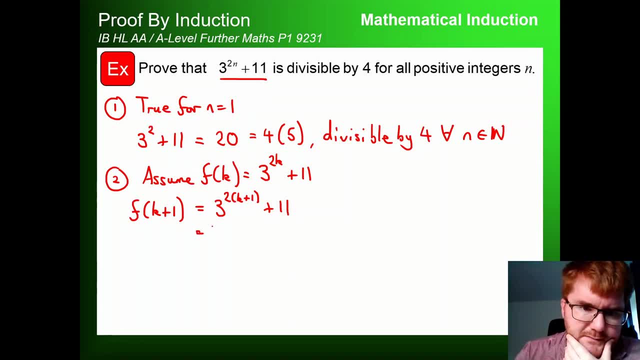 plus 11 and this becomes three to the power of 2k plus 2 plus 11. and remember, with indices we can separate this out, so we can write this as three squared times three to power of 2k plus 11. so again, just using those indices laws- they're very, very important- and of course three squared is. 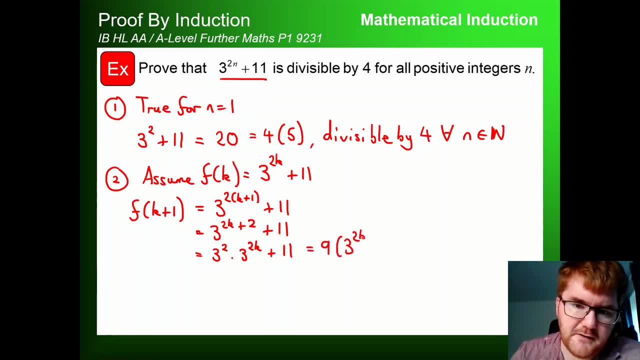 equal to nine. so we get nine, lots of three to the power of 2k plus 11. now the key step here is to actually consider- and this is going to help us show- it's divisible by four. consider f brackets, k plus one, minus f of k. you're thinking, why that particular expression? but you're going to see the. 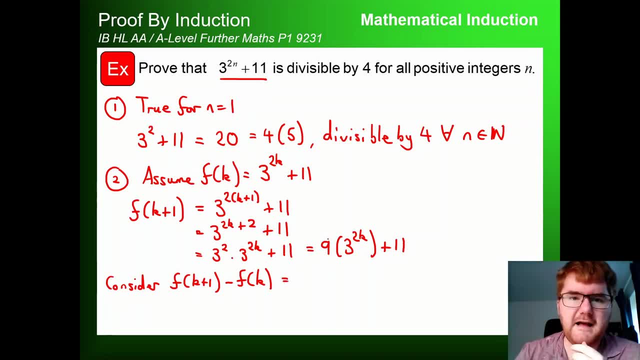 logic a bit later on. so if we substitute what we have in so far, we know, f of k plus one, is this expression so nine, lots of three to the power of 2k plus 11 minus f of k- this is where to be careful with negatives- so three to the power of 2k plus 11, if we simplify this out. 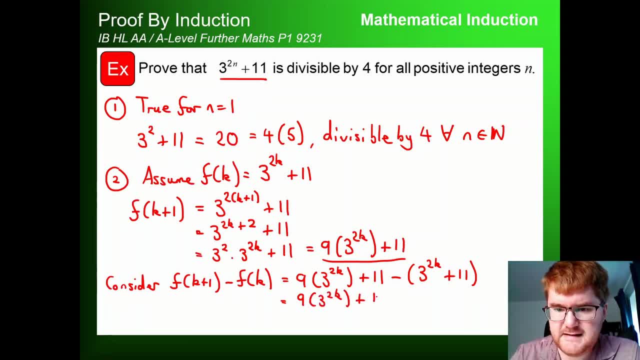 so we get nine to power three power 2k plus 11. that hasn't changed. remember, the minus applies to both things here. so we get minus three to the power of 2k minus 11. that means the 11 cancel, which is great, that's what we want. and now we've got essentially nine, lots of three to. 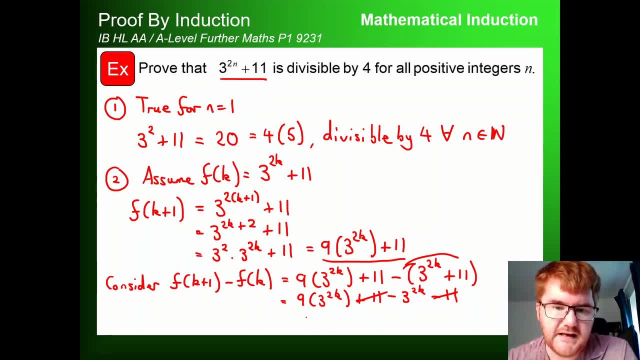 power of 2k minus one lot of three to power of 2k. that gives us eight lots of three to the power of 2k, and again this can be written as four lots of two lots of three to the power of 2k, so always. 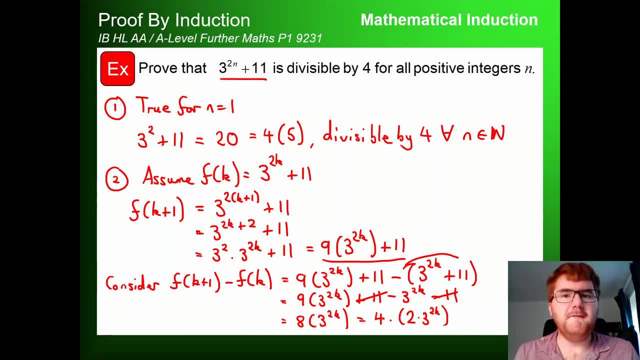 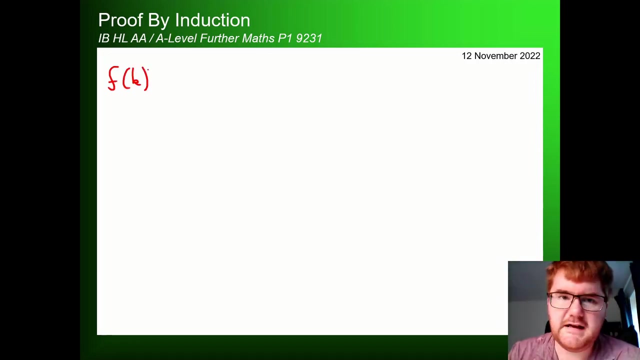 make it very clear to the examiner that is a multiple of four. yeah, so ie, it's divisible by four. so therefore this expression is four times something, so divisible by four. and if we write this out very cleanly, we get f of k. so what I'm doing? 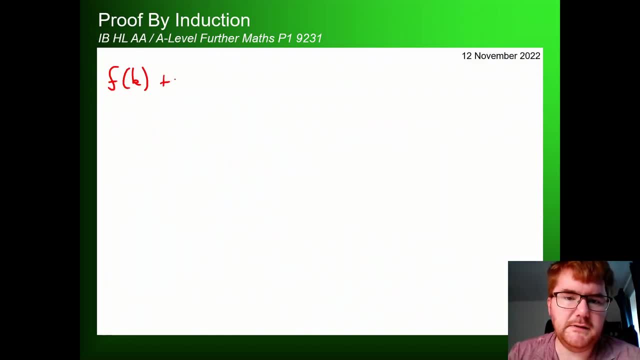 here is adding f of k on both sides. so f of k plus four- lots of three to the power of two, lots of three to power of 2k- is equal to f of k plus one. so this is divisible by four. this of course, by definition is divisible by four, because it's four times something. 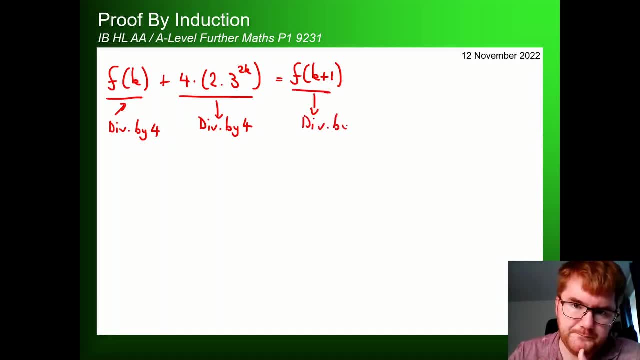 therefore this must be divisible by four, because they're equal. so n equals k plus one is divisible by four, and then therefore a statement is true for all. you can use the symbol for all, n, in the integers. so it's a similar thought process, it's just the algebra is a little bit different here. 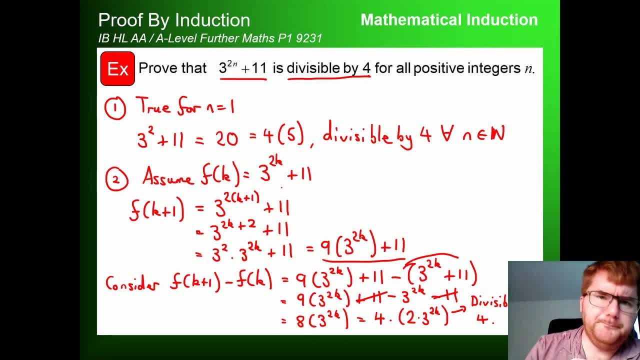 so you need to work through that quite carefully. so with divisibility, the first thing you do is step two. here you assume f of k is equal to your initial expression. you work out f of k plus one- it's going to take a little bit of algebra- and then you work out f of k plus one, and then you 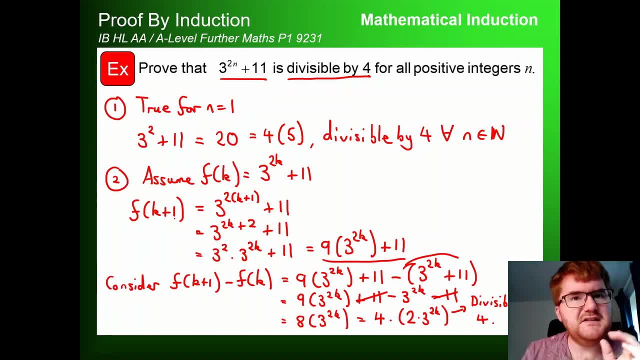 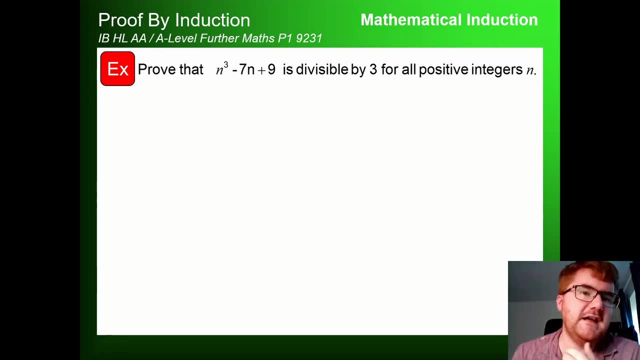 find the difference between them, and you want the difference to be a multiple of four in this case, and therefore it means then that f of k plus one will be divisible by four, and therefore is then true for all positive integers. okay, and on to another style of question here. so we've got. 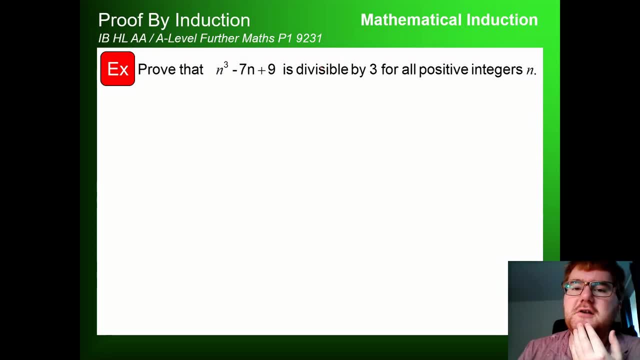 a cubic, n cubed minus seven, n plus nine, and we want to show it's divisible by three, this time for all positive integers, n. again we go through the same process. we want to find first of all that is true, for n is equal to one. so therefore we've got one cubed minus seven lots. 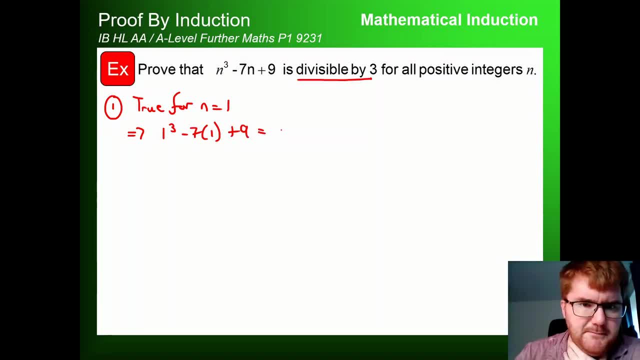 of one plus nine, so that becomes one minus seven minus six plus nine is three, and of course three is just three times one and therefore it's divisible by three. so the first step is always quite relaxing. again, i'm not going to try and trick you. it will be divisible by three, so you. 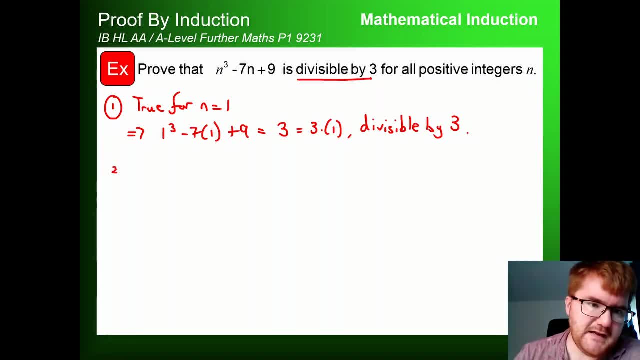 can see that it's going to be divisible by three or four or whichever number. so now we're into step two, which is the most complicated here. so we assume true, for n is equal to k. that means then f of k is equal to k cubed minus seven. n plus nine helps if i put k for each of the numbers. 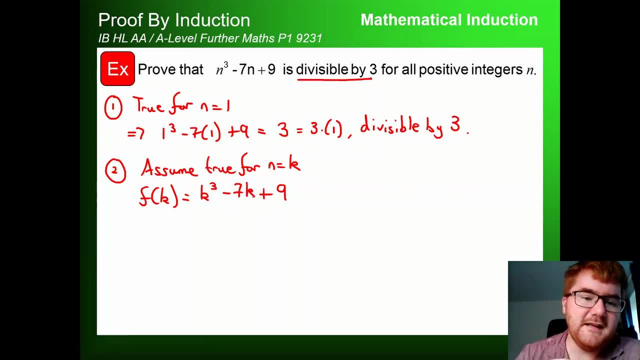 and i just change the variable halfway between theéf of k plus one. so we've kind of got a unique way of looking at some of this j hideout which is really really neat with when we minute the coordinate order, when we know that k is equal to one. so we simple to x minus theիx, we is less than it is equal to n. now 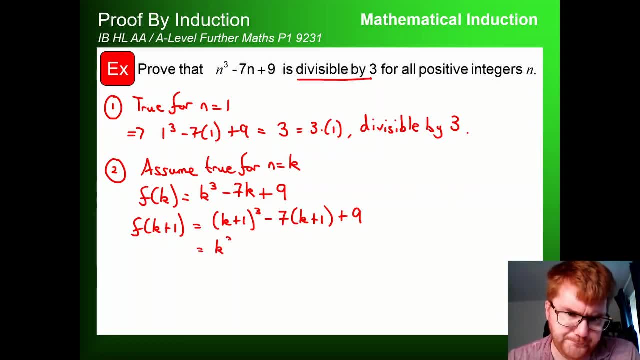 that this is our fundamental 임aflan subscript. we say this is f prime one. so that means we get k ن곱 plus n- mieux than to f시면 of k plus one. so wherever we see a k, we're going to put a k plus one. so you get k plus one cubed minus seven. lots of k plus one plus nine. now I've done some work on the binomial expansion here to work out this bracket again. i'm go through that in this particular video, but i'll just put the answer down. so we get k cubed plus three. lots of k neutral variety of s theoid. but we got only k. enough myself, not a lot of these, and I'm going to put that second value down right now and I'm going to. 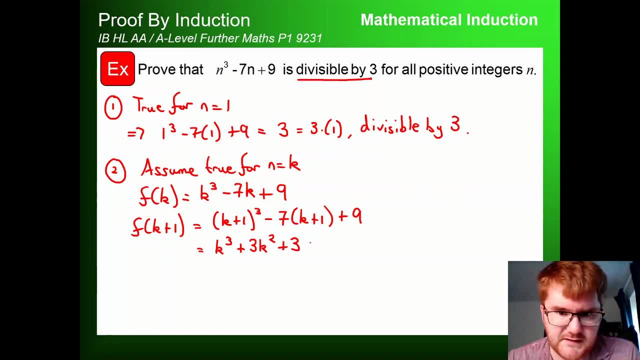 k squared plus three. lots of k plus one minus seven, k minus seven plus nine, and we want to simplify that down. so we get k cubed: uh three plus three k squared- that stays the same- minus four k- just being careful here- and minus uh one minus plus three. there we are, so we get the expression that we want. 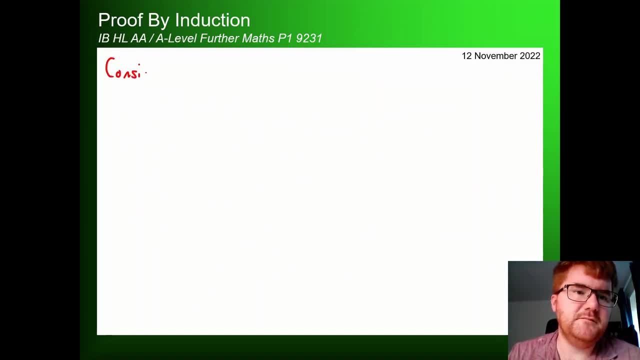 and now we want to consider- i'll do this on a separate slide this time- so then, consider f of k plus one minus f of k, so we take that expression. we just worked out k cubed plus three, k squared minus four, k plus three, and now we're going to take away our. 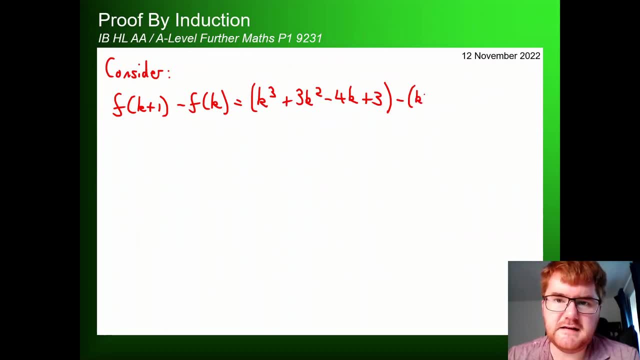 assumption, which is this step here. so minus k cubed, minus 7k plus 9. so let's see how this cancels. so the k cubes cancel. uh, the 3k squared stays where it is. we get minus 4, minus minus 7k. 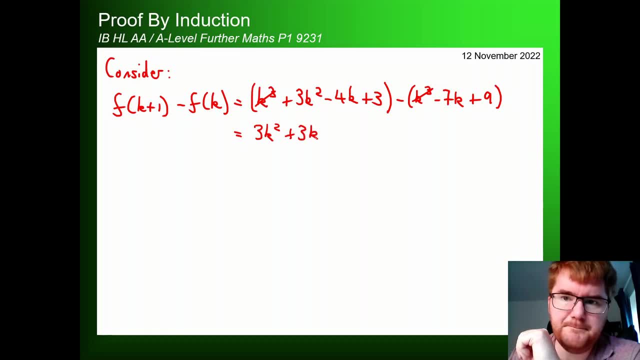 to be very careful there. that gives you plus 3k, and then 3 minus 9 is minus 6, and it's always a relief when you get to this part, because you can see quite clearly here it is divisible by three. so to show the examiner here, we then take a factor of three out of everything k squared plus, k minus.